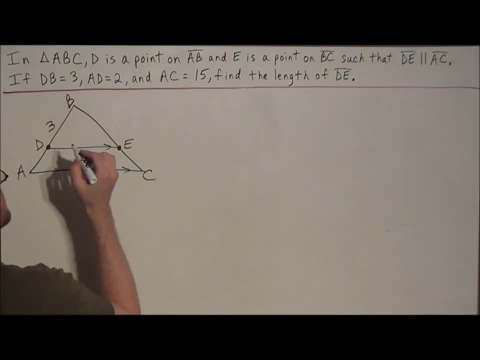 in the given information, we have that DB is equal to 3,, AD is equal to 2, and we have that AC is equal to 15.. And now, if the goal is to find the length of DE, we can call that side X. But now we need to think about all the given information. that was you know. 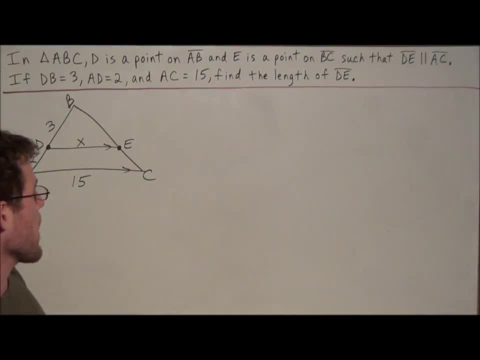 for us. If we're told that DE and AC are parallel, this is usually going to indicate that we're going to have congruent angles. So we could say right away that angle A and angle BDE are congruent because they're corresponding. 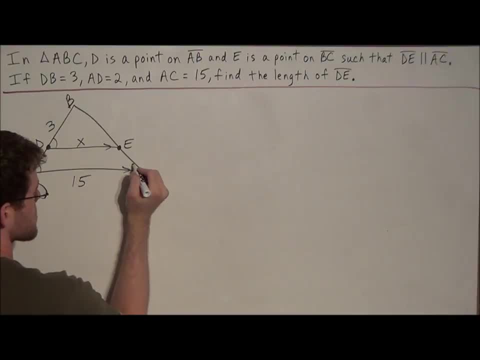 Likewise, a similar argument tells you that angle C and angle DEB are also congruent. So this tells us that we have two similar triangles. We have triangle DBE is similar to triangle ABC, and if we wanted to justify this, we could say by: 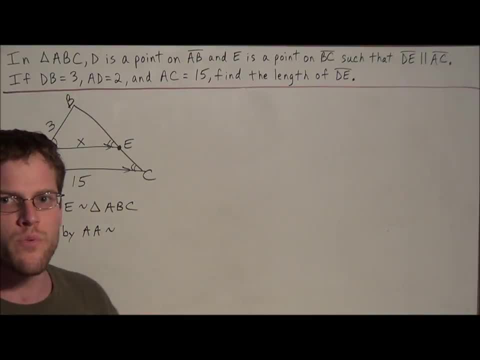 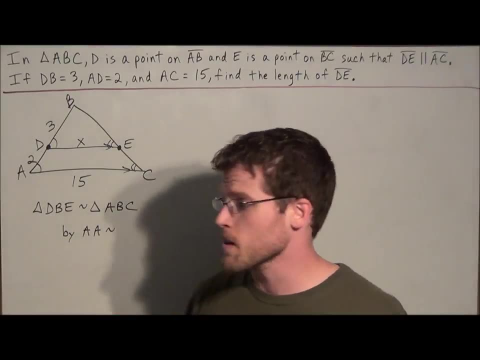 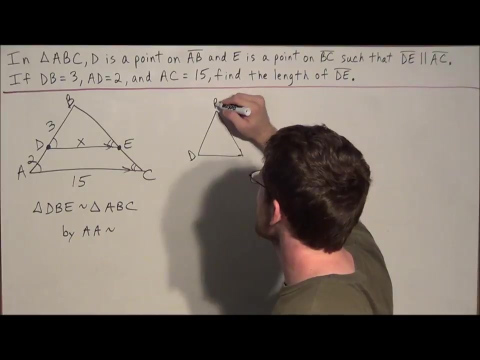 angle-angle similarity. We're not going to write a formal proof, we just want to solve this problem. But the strategy is, since we have these two similar triangles, we want to draw them separately. So we start off. we have triangle, we have triangle DBE and we can fill in the size that we know. We 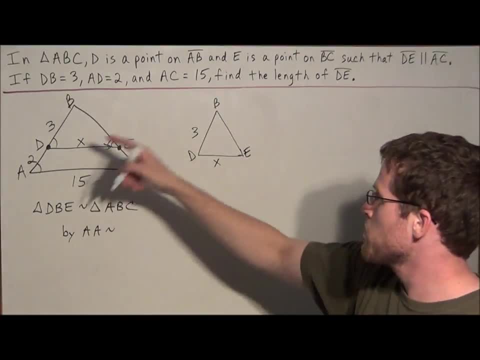 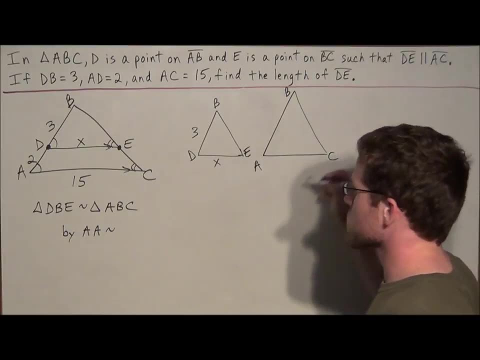 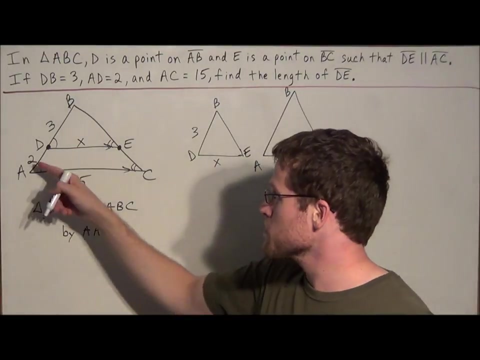 We know that DB is 3,, DE is X. and now the big triangle, ABC. we know that side AC is 15, but now let's just do all the work right here: AB. we can find the length of AB by adding up these two smaller segments. 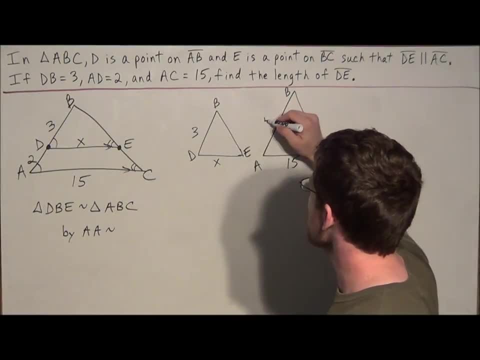 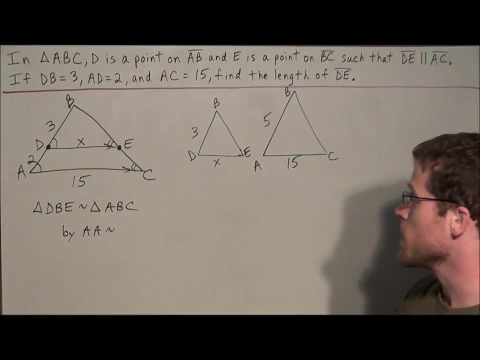 We have: 2 plus 3 is 5, so the length of AB is equal to 5.. But now that we have these triangles lined up, we can set up a proportion and find the value of the missing side. And now the strategy for this. we can set up many different ratios, as long as we're 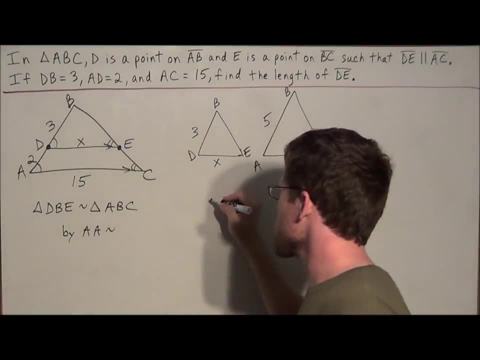 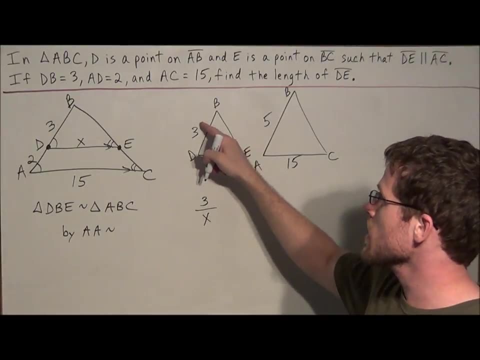 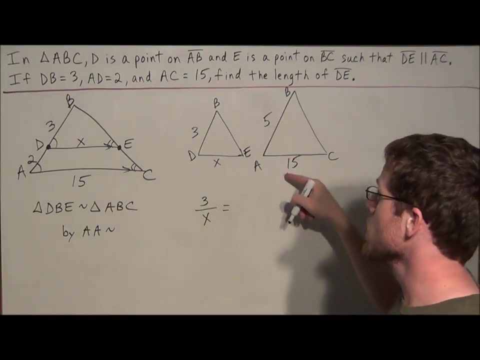 consistent, And what we mean by this is that, let's say, we set up the ratio 3 over X, We're comparing the side on the left and the bottom. So we're comparing the left side to the bottom or the base. So when we set up the ratio in this triangle, we need to compare the side on the left to 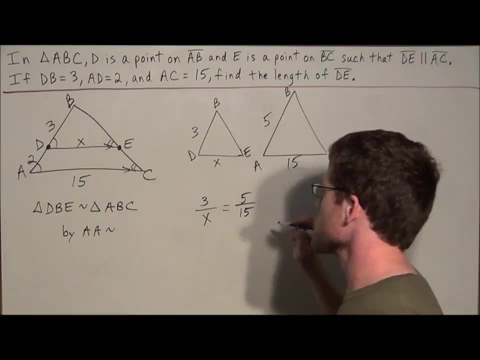 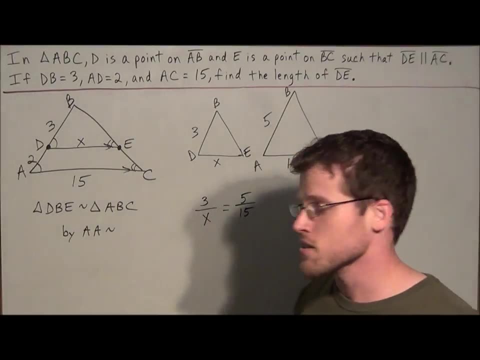 the bottom. So we're setting up 5 over 15.. So just once again, we're comparing the left to the bottom. So 3 over X Equals 5 over 15.. Now, at this step, all we need to do is cross multiply.